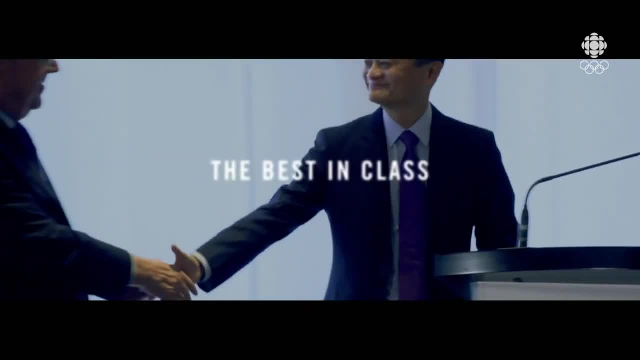 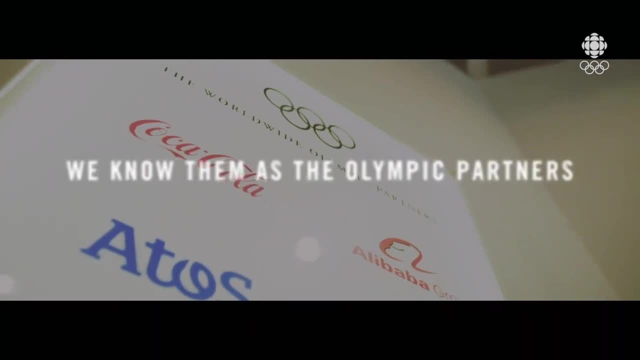 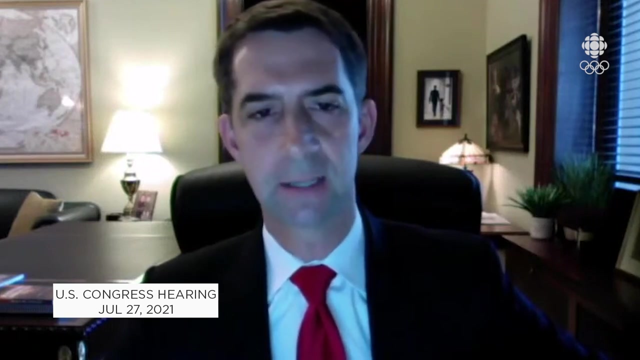 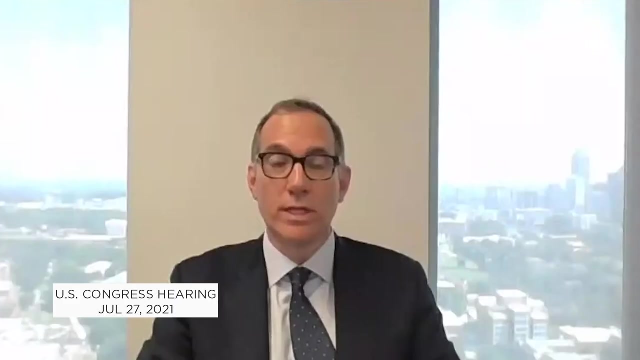 So can you tell me why Coca-Cola doesn't have a say in whether it sponsors the Genocide Olympics next year? Senator, what I stated was that we do not have a say in the selection of the host city, nor on whether an Olympics is postponed or relocated. I mean, we're all waiting with. 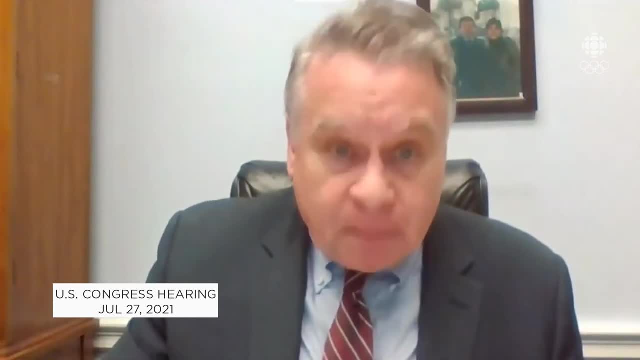 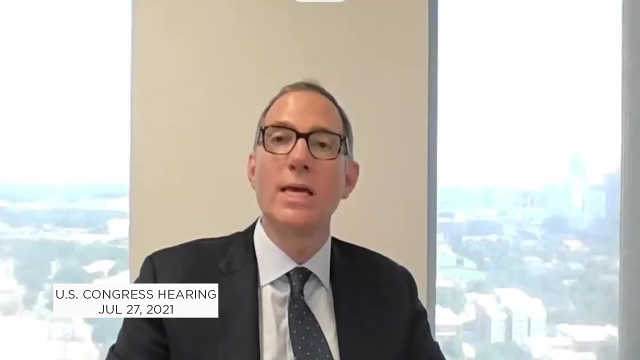 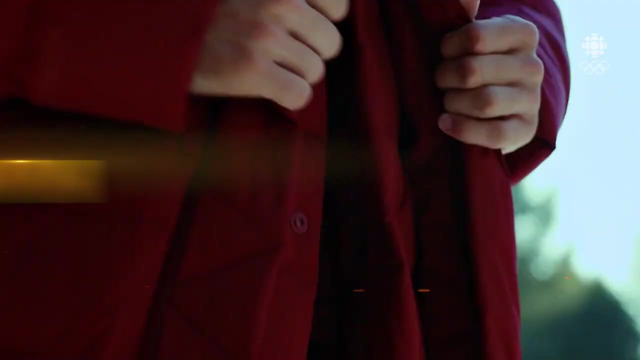 bated breath for all of you to say: move the Olympics. The Beijing Genocide Olympics need to be moved. Can't you say that We don't make a decision on the host location, but we work on the human rights aspect and there has been progress in the space For advertisers. the 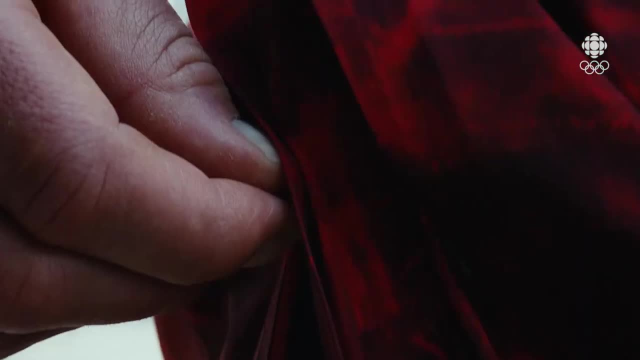 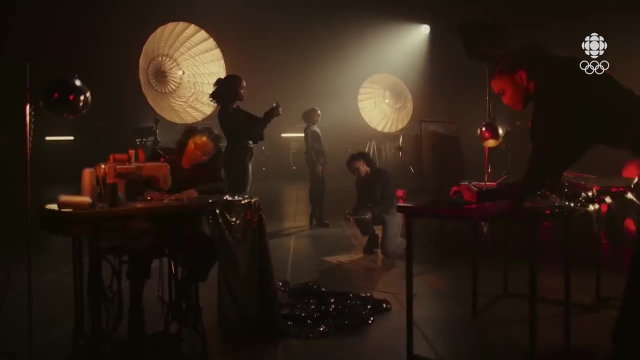 Olympic Games is the holy grail of marketing. For the IOC it means billions of dollars as companies clamor to be part of the traditionally feel-good event. But these Beijing Olympic Games are different. Many companies are taking a low-key approach, balancing a fine line between 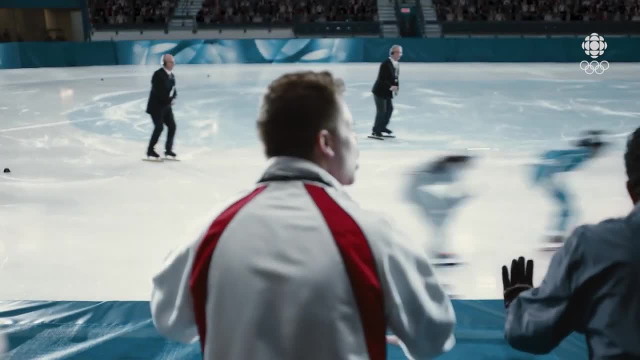 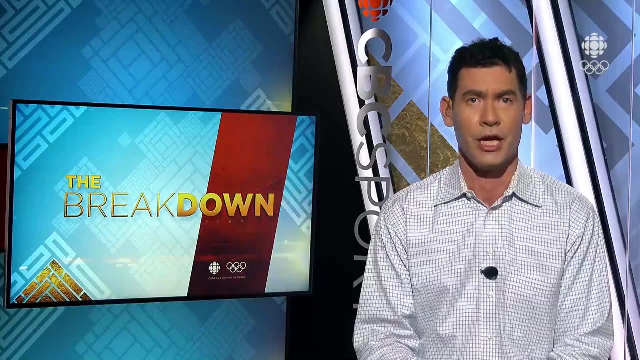 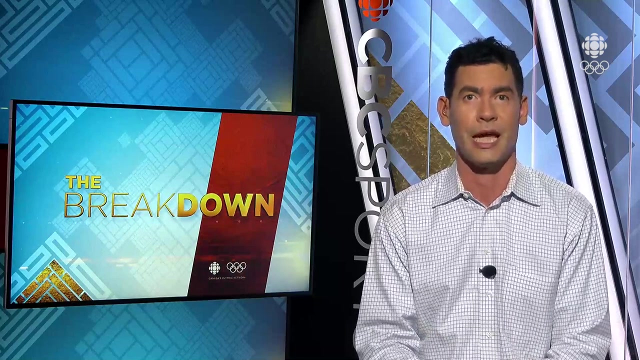 their investment and anger around China's human rights record. For more on this, I'm joined by Dehi Kwok, a professor of sports marketing at the University of Michigan. Professor, we usually see a lot of splashy ad campaigns both leading up to and during the Games. 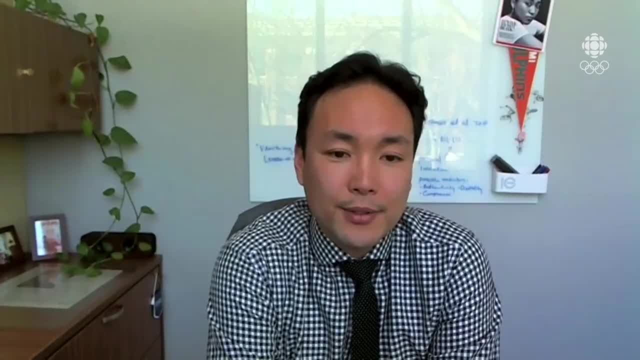 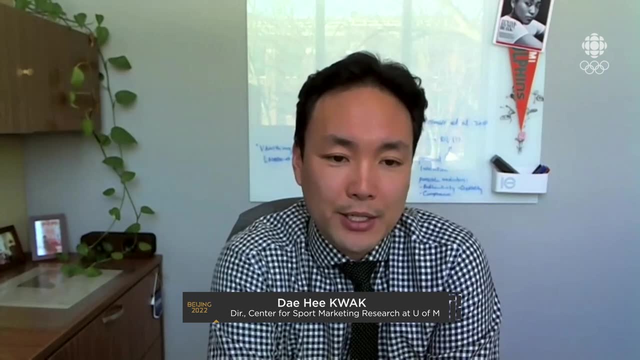 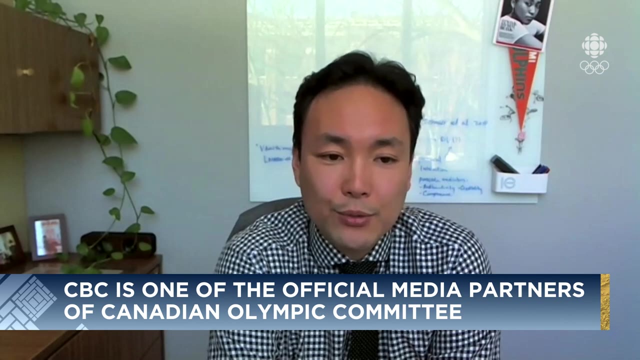 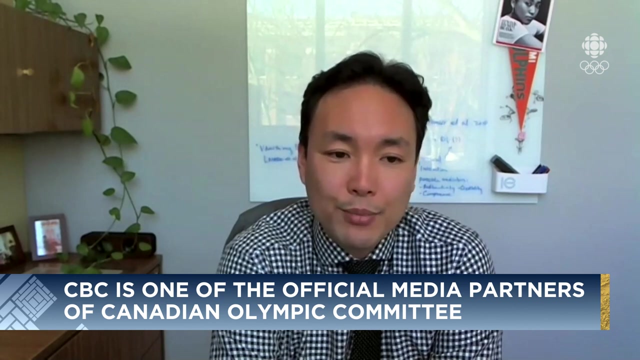 but they're very muted this year. Why In China they have different information about what's going on in Xinjiang area. So that is putting sponsors in a very difficult situation. to what do we do? Do we either boycott or do we pull out, or do we just ignore what's going on, Which put a lot of pressure on sponsors. So 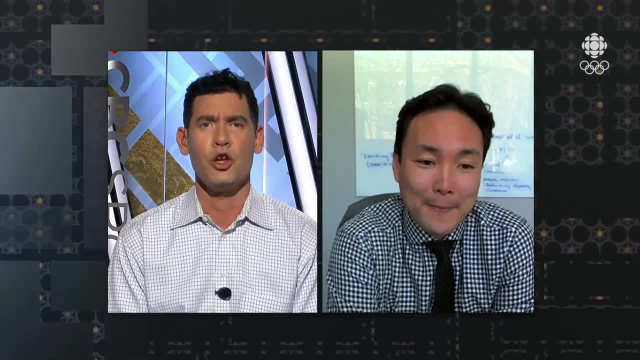 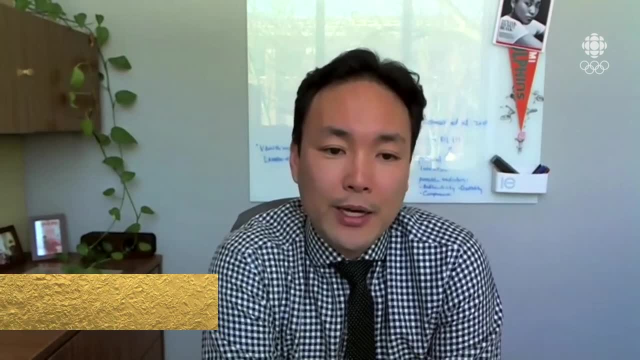 staying muted might be the best course of action. for now, No major sponsor boycotted these Games. Why do you think that is? Sponsors are not in the Dependent from what's going on And they have to really navigate through. what do we do? And 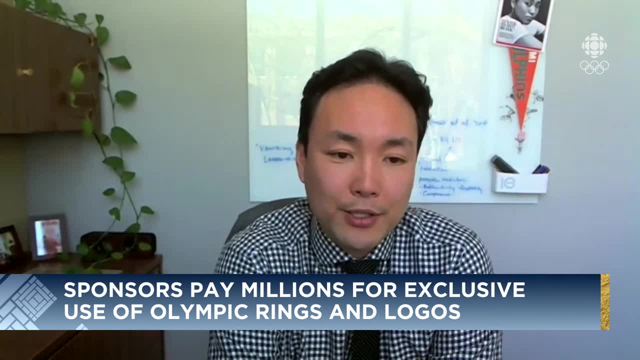 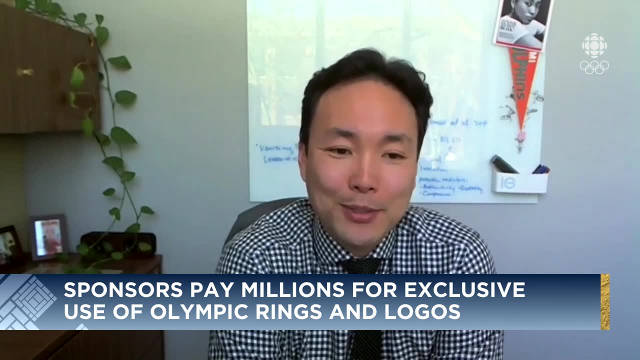 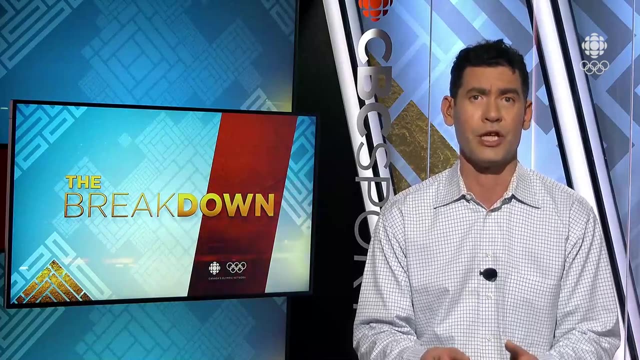 if there will be a potential backlash from Chinese market. So you don't want to upset the Chinese market for sure, Because if you learn from the past, there has been a retaliation from the Chinese government as well as Chinese consumers. Are advertisers willing? do you think to risk alienating their Western customers? 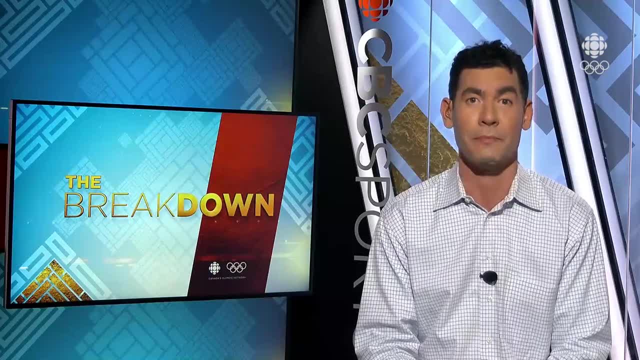 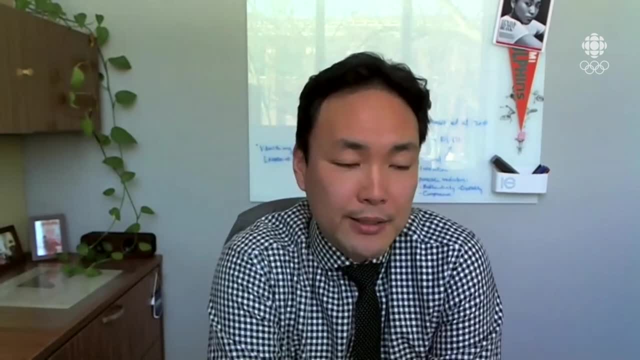 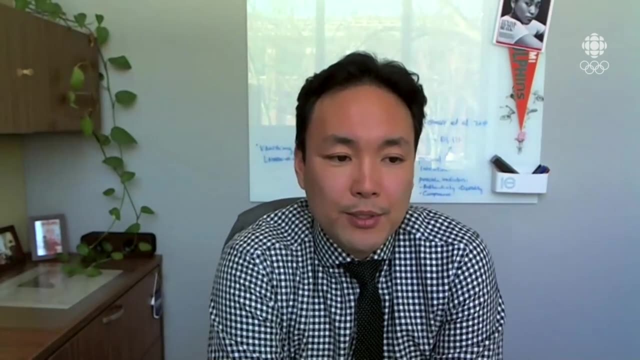 in exchange for accessing the massive Chinese market. That's what's going on with Coca-Cola, just, for instance, in domestic market. So they focus on rather host city, for instance, because it's a celebration in China right now, with Beijing being the first time hosting the Olympics, And Coca-Cola is doing a lot of activations in China Getting 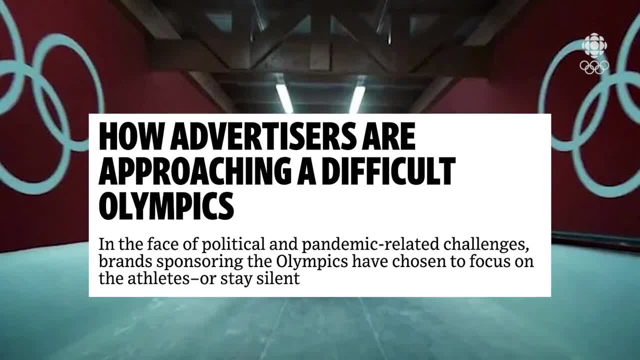 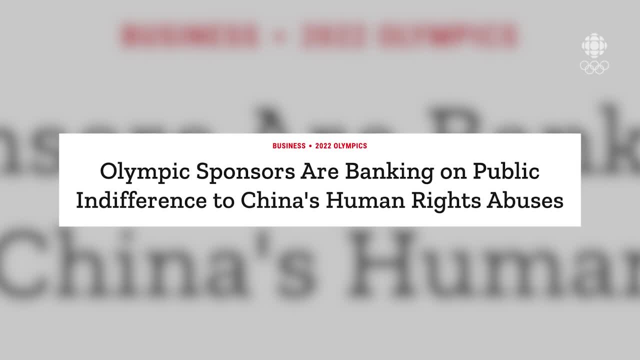 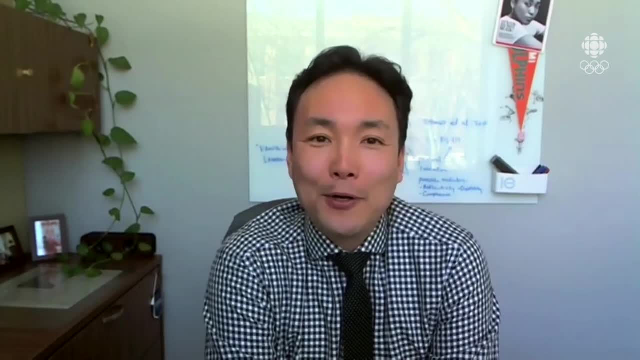 Chinese market involved with the Olympics. I think this would be a great opportunity because they are the hosting nation of the Olympics. So it's unfortunate that this, the current climate and what's going on- Just not allowing this companies to openly or really celebrating these Olympics in both a home market as well as in Chinese markets. 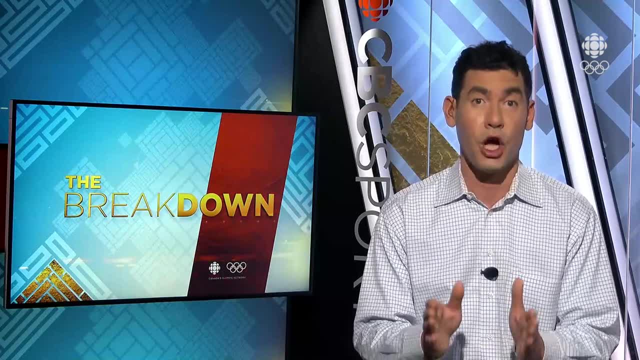 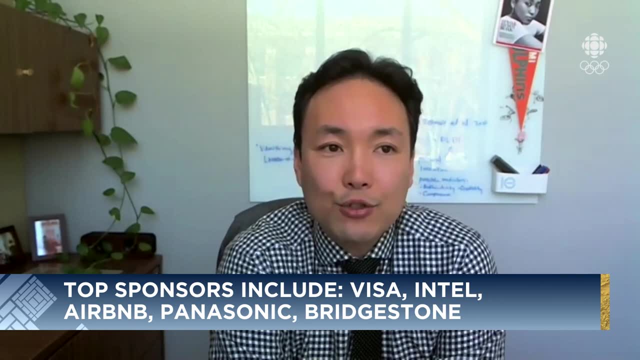 Usually around the games we see ads that kind of play off the culture of the host nation, but not really this time. Why do you think that is? I think the advertisements are trying to portray why people stick with the Olympics or why people tune into the Olympics, So I'm not really sure. if that's the case, I think the 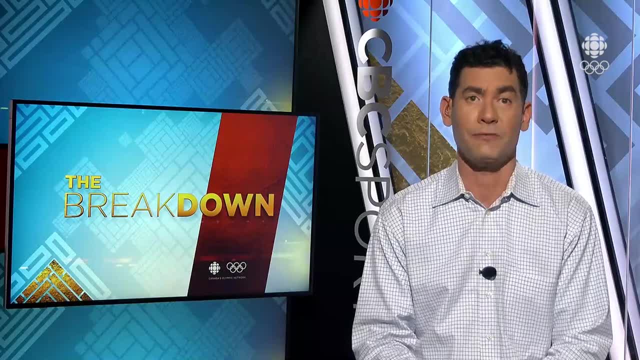 entry in the headlines. I think it's very close. So I think the entry in the headlines, I think I think the entry in the headlines, I think it's very close, So I think it's very close, So I think. Will advertisers face any blowback in the West for their association with these games? 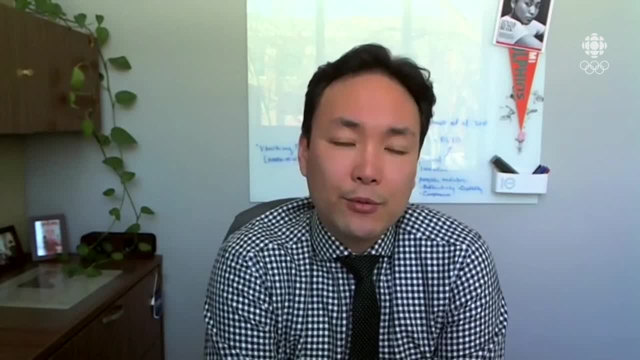 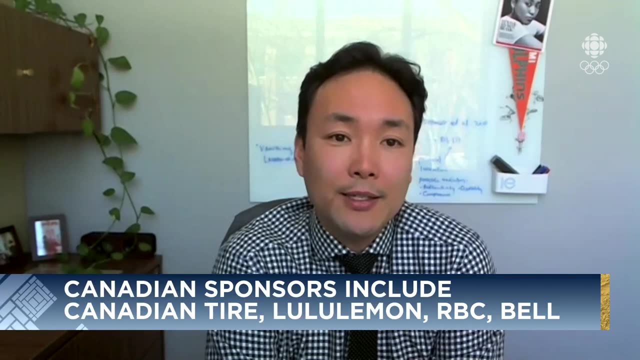 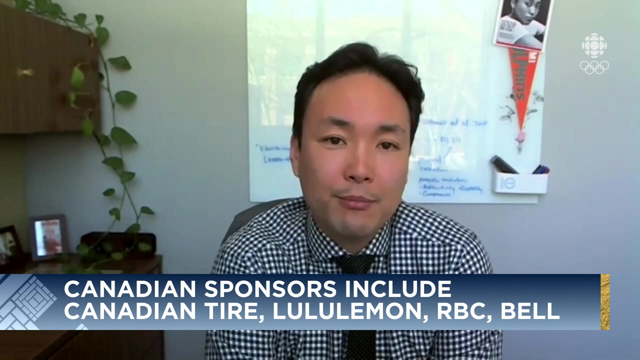 You know you will have some glitches here and there with what are you doing? Why are you so silent? But the brands will move on And the Beijing Olympic is not the entire marketing platform that they rely on, So I think it's more of a PR issue from the Western media standpoint. 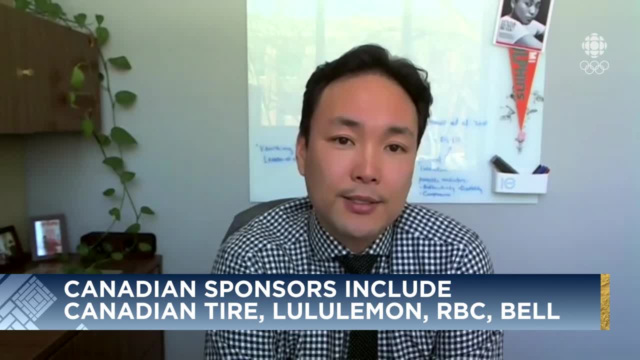 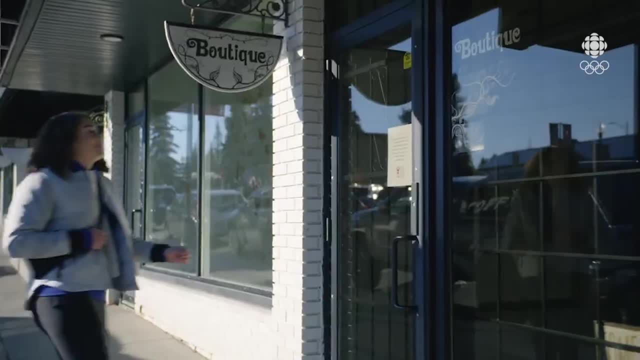 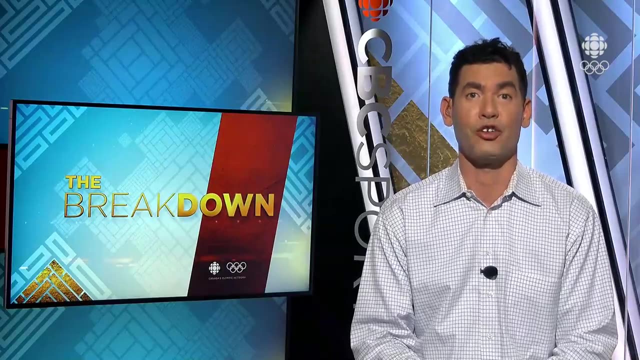 But if you look at Chinese market, it can really hurt the bottom line of the business. So if we boycott or if we take a stance, that's what the corporations would fear more about. In North America, one of the leading critics of corporations linked to these Olympics 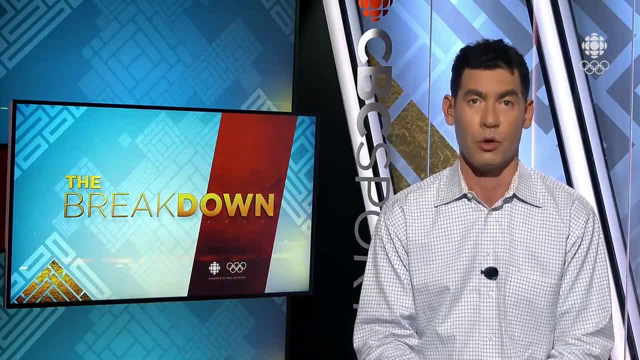 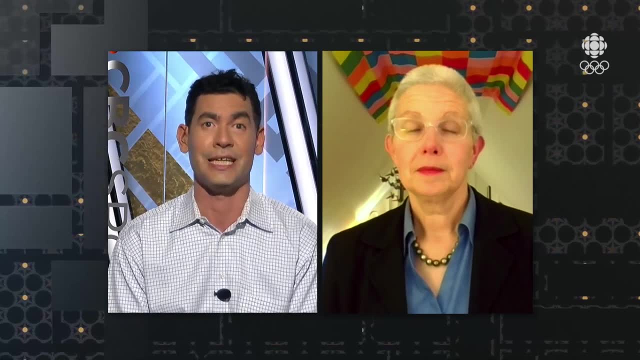 has been Sophie Richardson of Human Rights Watch. We reached her in Washington. Sophie, you wrote a letter to the top Olympic sponsors asking what kind of diligence they did around China's human rights record. Tell us about the letter and what kind of response did you get? 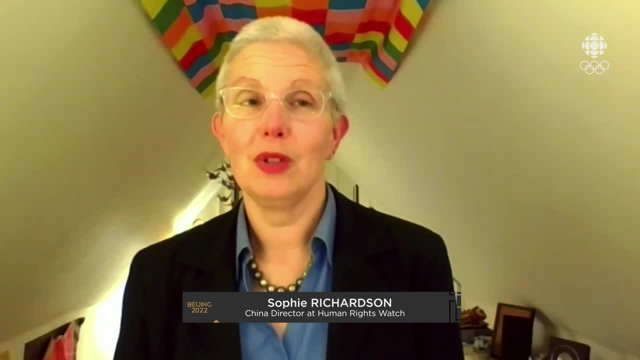 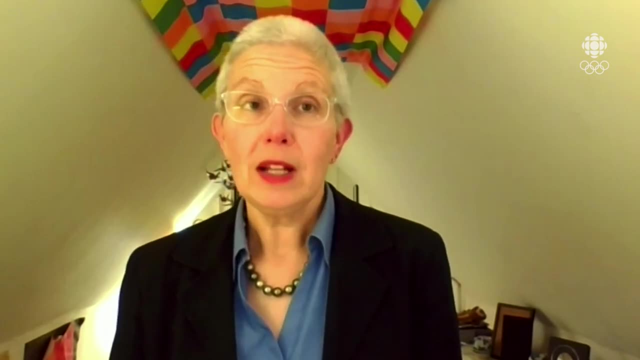 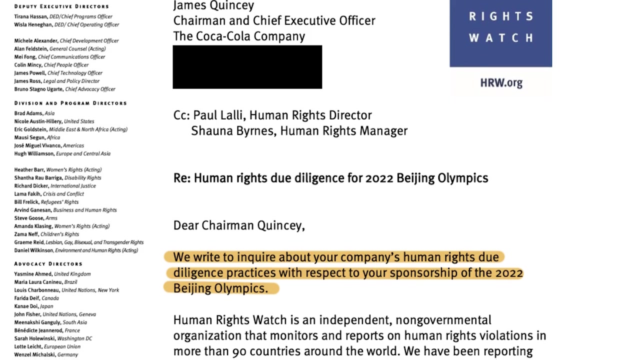 Sure, It's now been almost a year actually since we wrote to these top tier sponsors of these particular games And we asked them really a very simple question: What human rights due diligence had they done around their sponsorship of these games, Meaning, had they asked themselves questions about reputational risk? 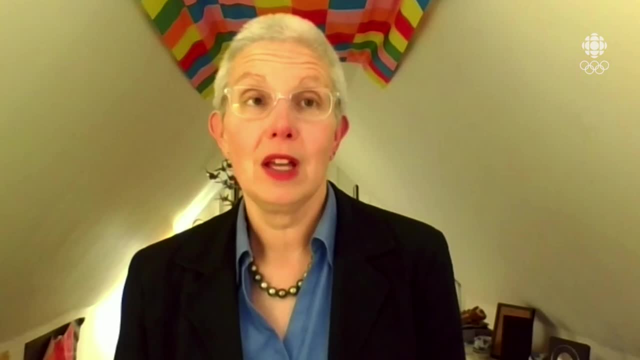 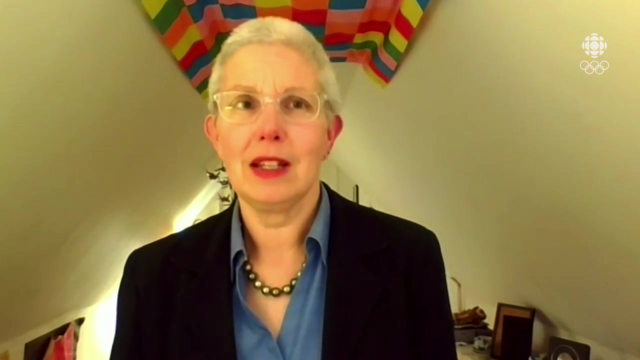 Were they sure that their supply chains are free of problems with respect to forced labor? Now, these are all standard affirmative responsibilities Companies are meant to fulfill Under a set of United Nations guiding principles, And the fact that none of them really gave us an even remotely meaningful reply. 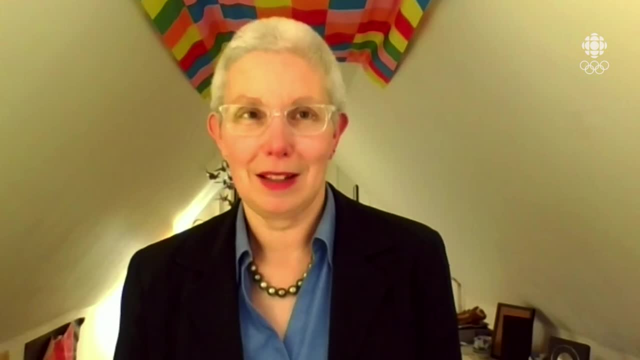 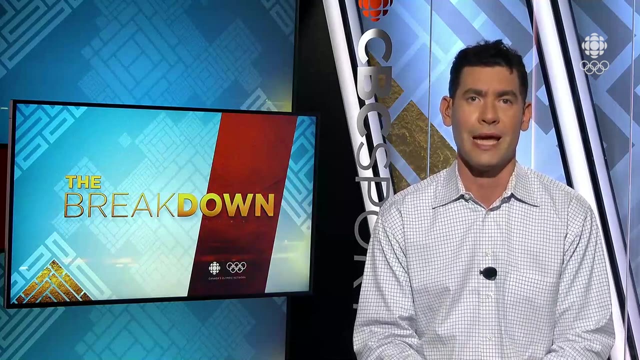 I think you know can be taken to mean that either they didn't do that kind of homework or they're not going to talk about it. Sophie, what are governments doing to make companies more accountable for doing business in China? There is now binding legislation here in the United States. 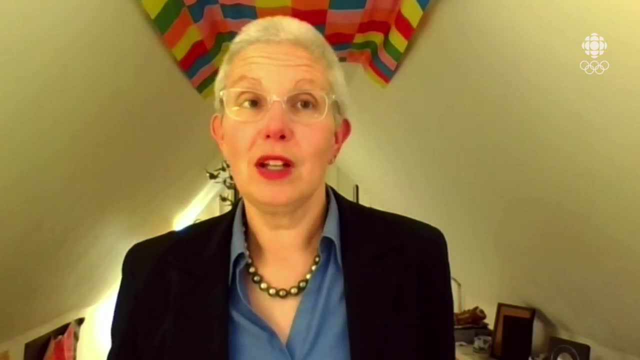 and that other governments, including the European Union, are considering, that will require companies importing goods, at least from Xinjiang Uyghur region, to show that they're not made using forced labor, Because these voluntary standards that companies have been asked for years to fulfill. 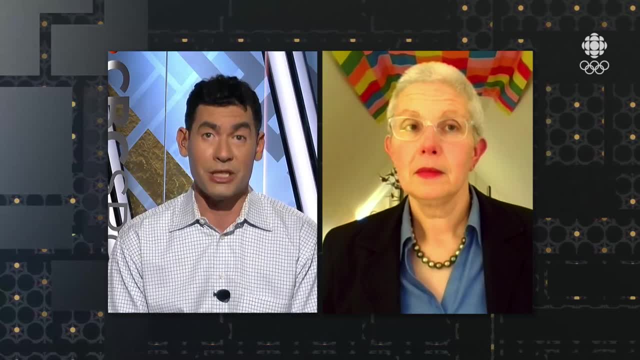 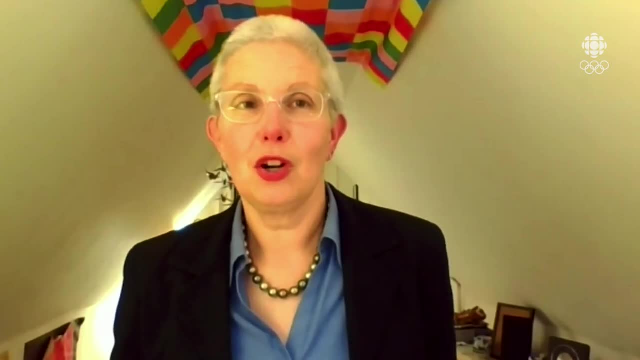 haven't really worked. As you pointed out, companies have been remiss to talk about their Olympic involvement. Why do you think that is? Well, I think they're trying to make sure that they don't get caught in the crossfire, essentially between two different sets of standards, right? 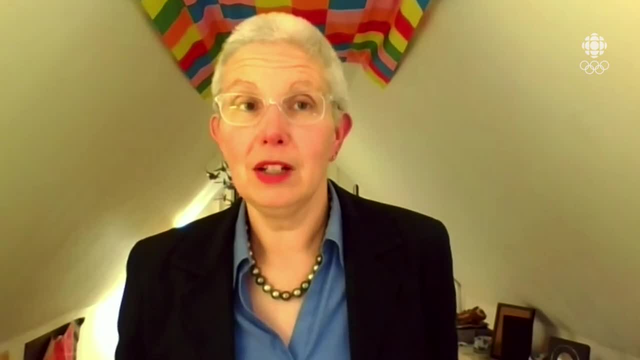 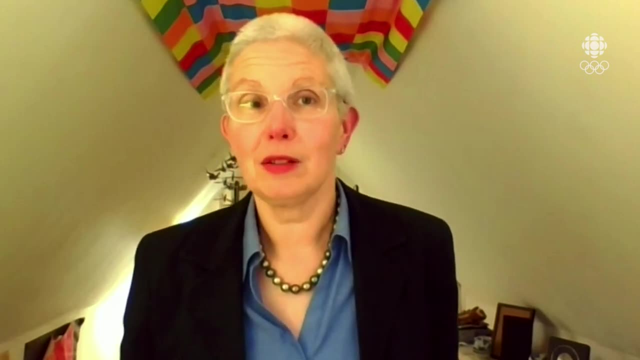 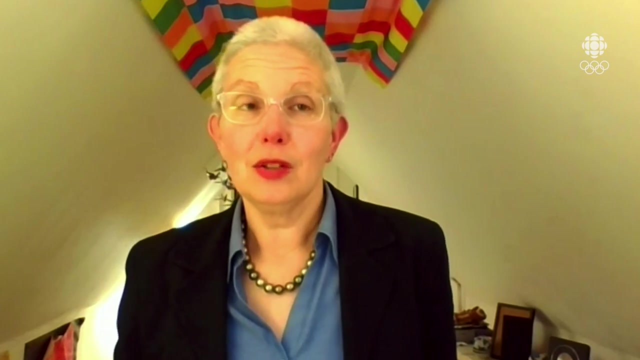 And that's just the way it is. And that's just the way it is. The Chinese government has not been shy about punishing foreign companies they perceive as being critical of their human rights record, particularly around Xinjiang, for example. You know, when, externally, companies are increasingly under pressure. 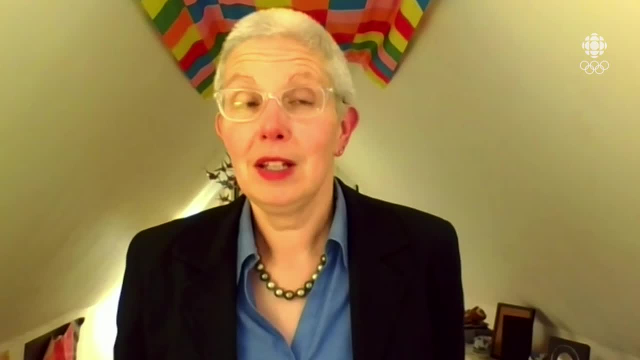 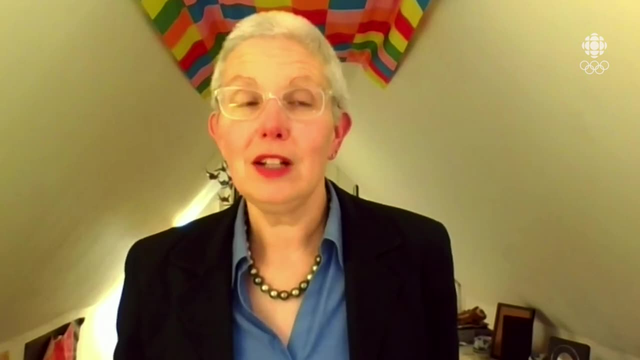 including now by way of the Uyghur Forced Labor Prevention Act in the US, you know, not running afoul of that legislation- And these two things really do pull in different directions and increasingly companies are going to have to make a choice about, you know, how they're going to do business. 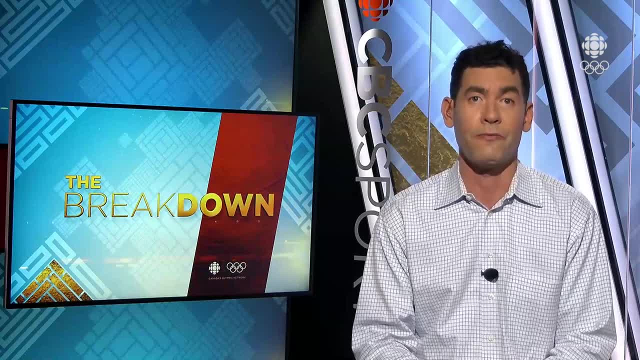 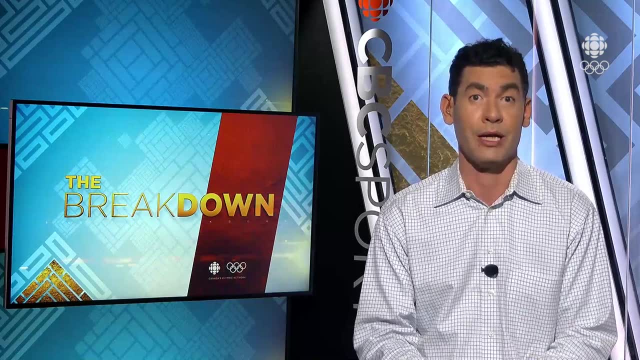 Sophie, many of the companies, including Coke and Intel, were called before Congress and grilled on their involvement in these Olympics. They basically said this doesn't lessen their commitments to human rights. And, by the way, we don't choose the host. Can they have it both ways? 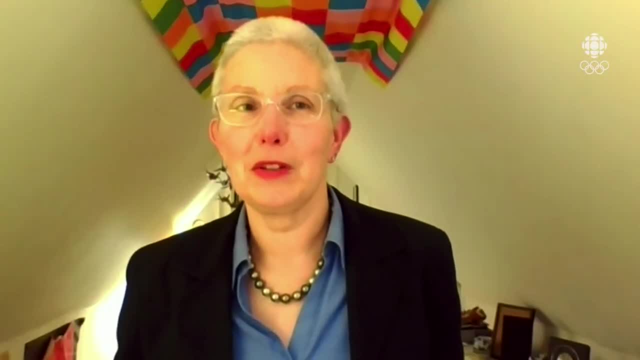 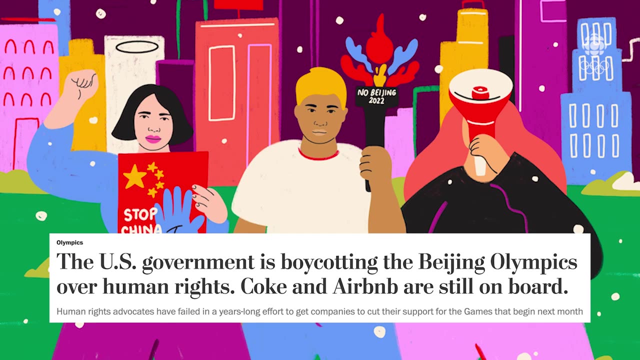 Well, you know there's nothing written in stone saying they have to sponsor Olympics for starters. You know many of these companies hold themselves out as being great defenders, you know, of ESG rights or human rights. You know Coke recently was was very visible in a discussion here in the US.